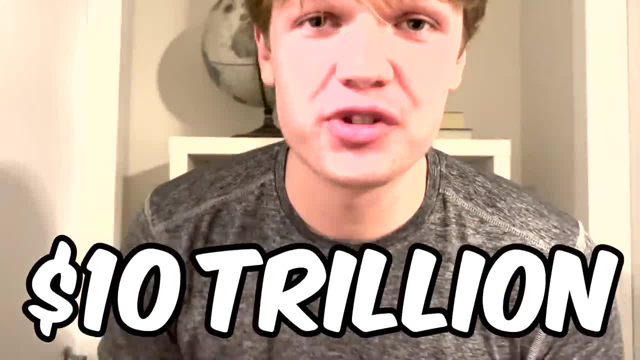 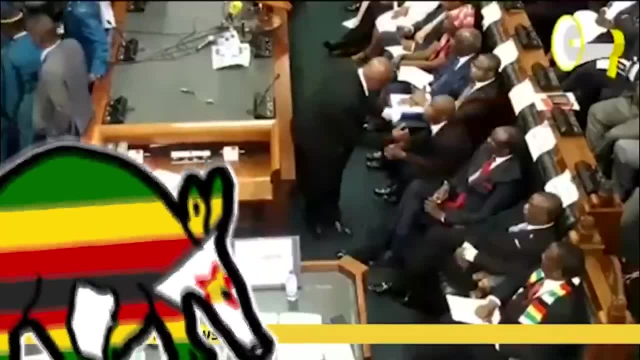 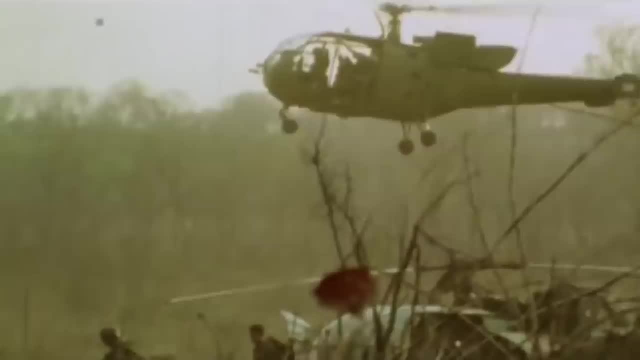 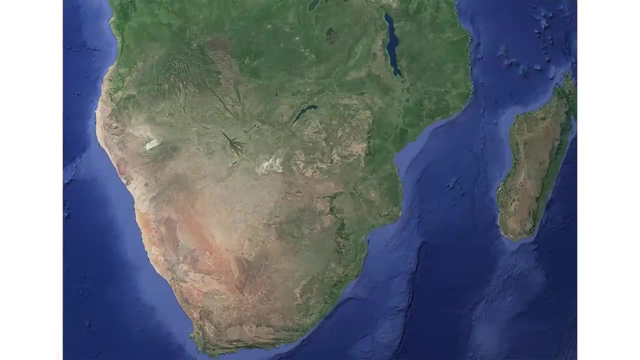 In this video, I'm going to be giving away 10 trillion dollars to a random subscriber. Zimbabwe dollars, baby, We are not gay. First, let's look at modern Zimbabwe, Sitting in the rump of Africa. Zimbabwe is made up of: 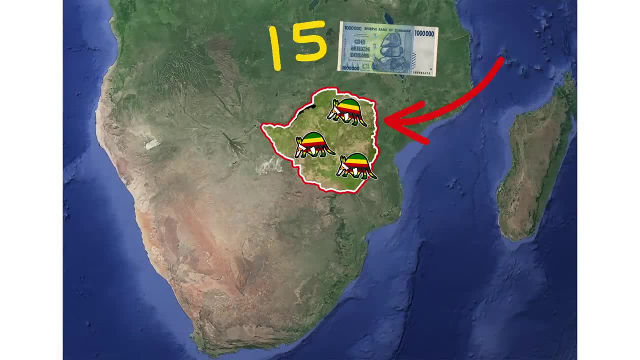 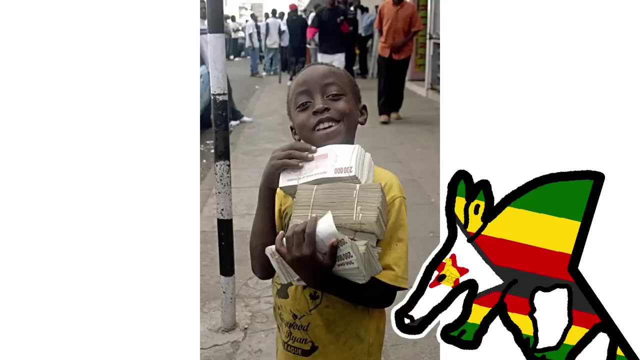 these borders and sitting at a population of about 15 million. on this rather boring piece of land, the nation does not produce a whole lot of anything. How do they make their money then? For two-thirds of the country they don't really. They just farm. 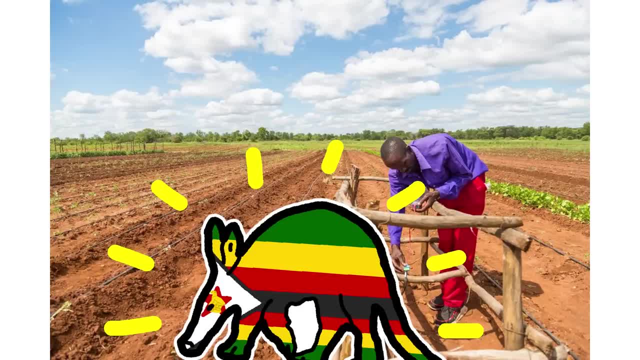 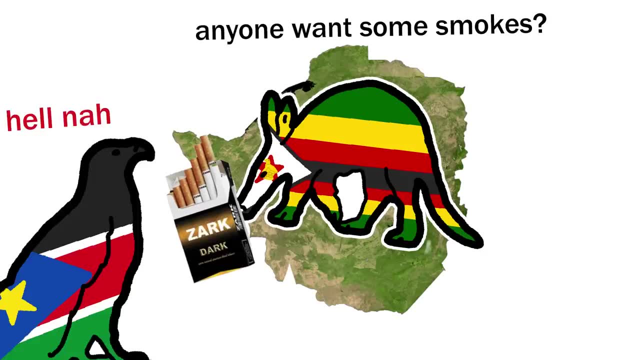 usually at the sustenance level. That means they're self-sufficient, right? No nation is really self-sufficient, not even you. So the rest of the nation can trade to make up that difference. But wait, Zimbabwe is a landlocked nation. They need to get through both. 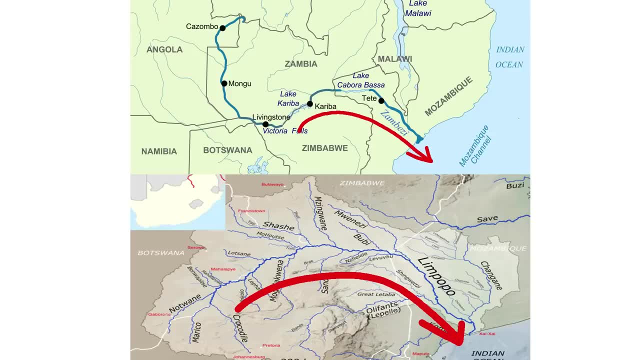 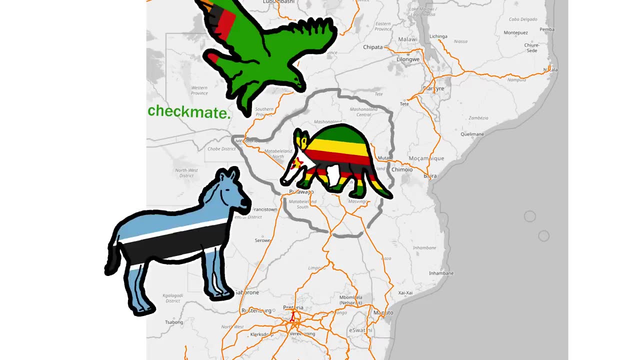 South Africa and Africa And Mozambique through these rivers in order to ship their goods off, That is, unless they move it by train, still needing to rely on these two countries plus Zambia or Botswana now, And African borders are notorious for corruption and usually a little extra side. 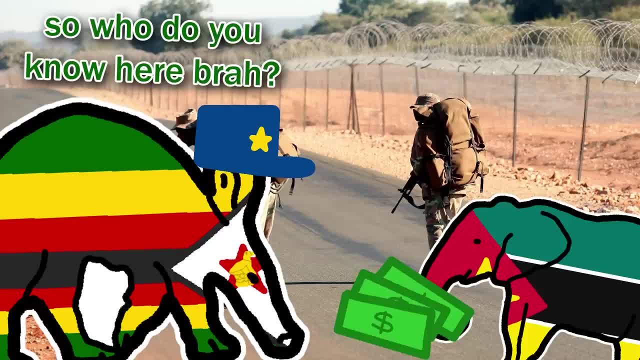 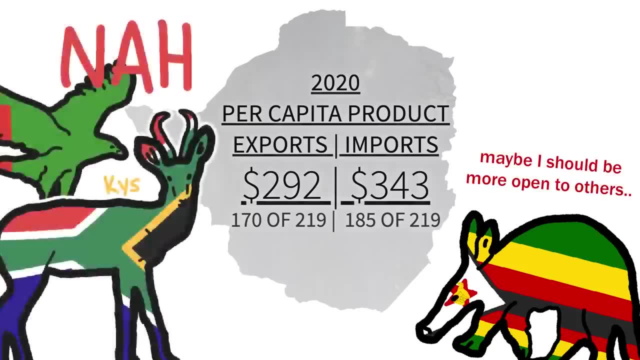 cash is given to the officer when crossing Meh. Just think of it as a tariff. This all leads to Zimbabwe having one of the lowest rates of trading per capita on earth and, as you'll see later, they didn't keep great relations with any of their neighbors, Although, if you included smuggling in their trade. they would have been able to get a lot of money off of it, But Zimbabwe is not a landlocked nation. The answer would be a lot higher. What could they possibly be smuggling? Marijuana, Meth, Heroin, Nah, More like flour gold and just a dash of cocaine. 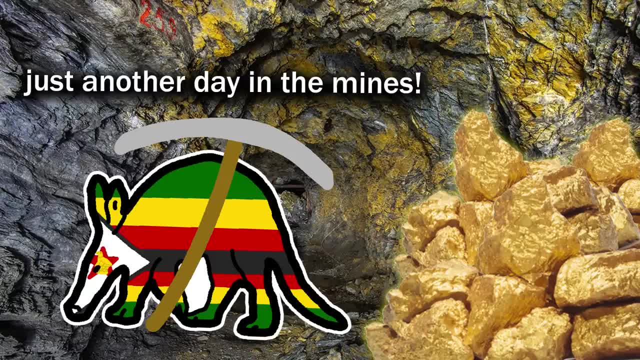 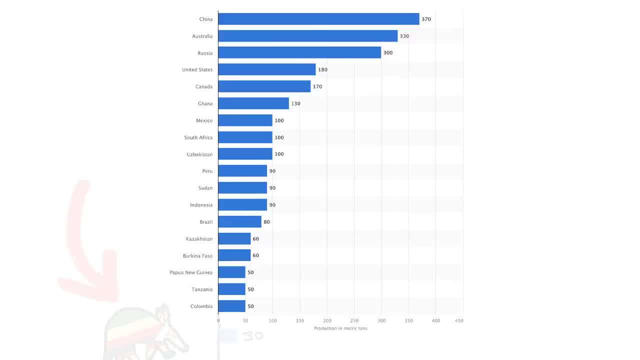 You might have heard, it's because Zimbabwe is one of the largest gold producers on earth. I mean, it makes up half of their exports. Of course they produce a ton of it, But no, the gold production is relatively small, with only about 30 tons produced a year. 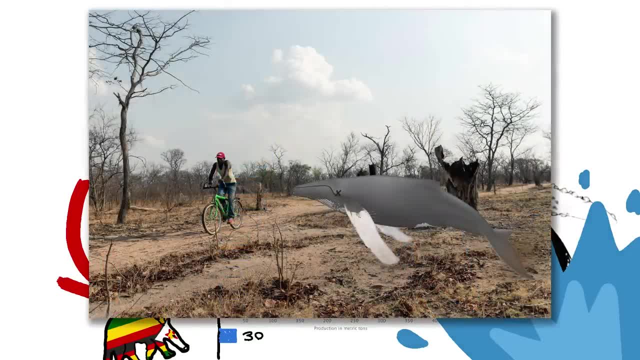 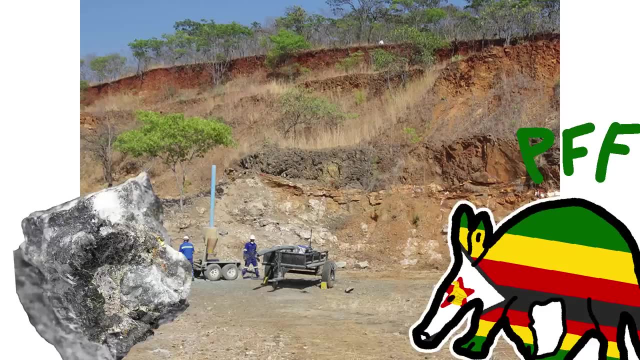 That's about the weight of a humpback whale, Or a dead humpback whale, because they don't have any oceans in Zimbabwe. Real great exports, huh? What they do have instead is platinum, chromium and some lithium. Mining is Zimbabwe's big thing. It's the whole reason it was colonized. 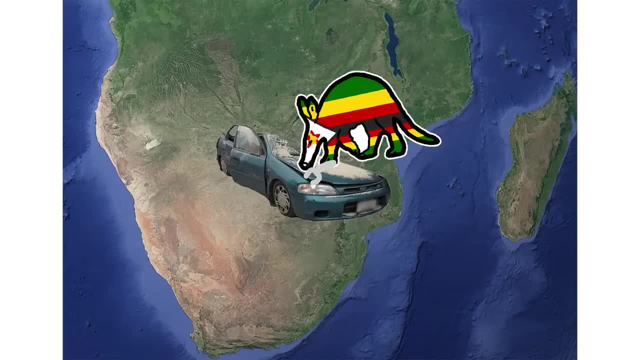 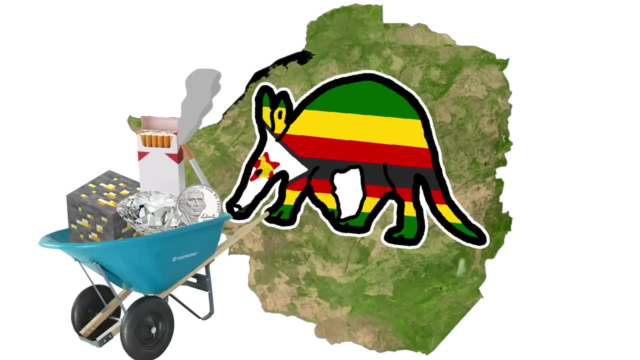 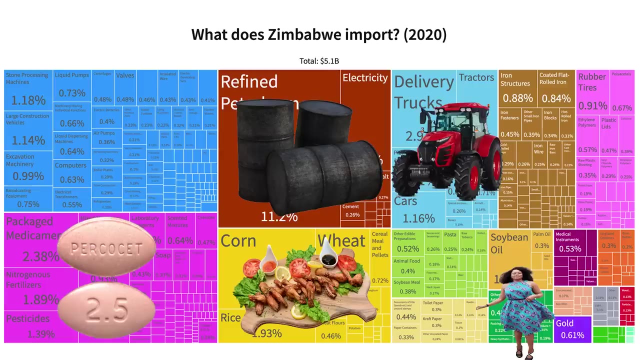 in the first place. Pretty much every other industry is too uncompetitive for Zimbabwe to fight even its neighbors in, So they export things like gold, diamonds, nickel and some tobacco for good luck, and import things like everything- At least everything you need for a modern country: Food, energy, chemicals, vehicles, clothes, industrial supplies. I don't want to go on, especially since they still barely import anything. This low level of trade makes them so vulnerable to swings in the domestic market, which means if times are good they're pretty good, And if times are bad they get worse than most other nations do. They can't minimize. 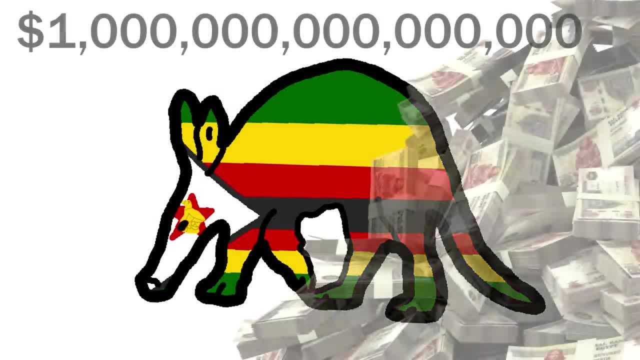 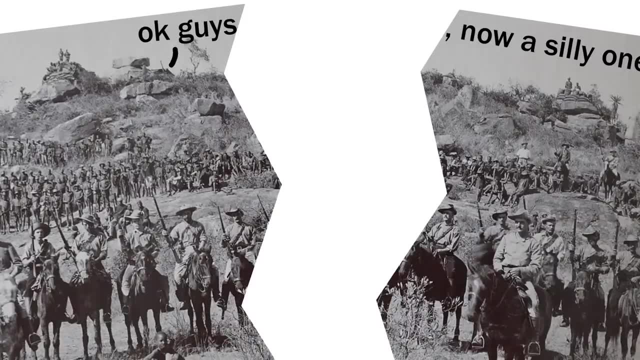 any shocks with outside trade. Let's get to the blunders then. First mistake these guys. Look how friendly they are. Just imagine being posted up with the boys in a foreign land. Only one issue: there are still these fellas living here, the Ndebele. So by the 1880s there was an. 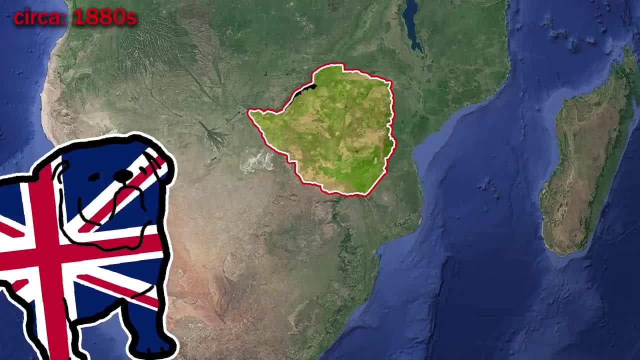 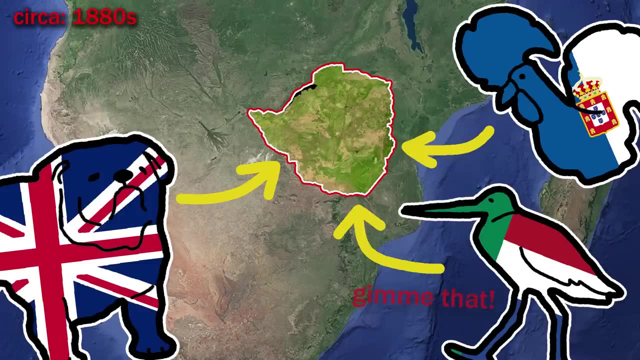 old African standoff. This is basically how it went. The British said: I want this land. Then the Portuguese came in and said: I want this land. Then the Boers came too and said: I want this land. And then Ndebele said: what the hell, This is my land. So the British told: 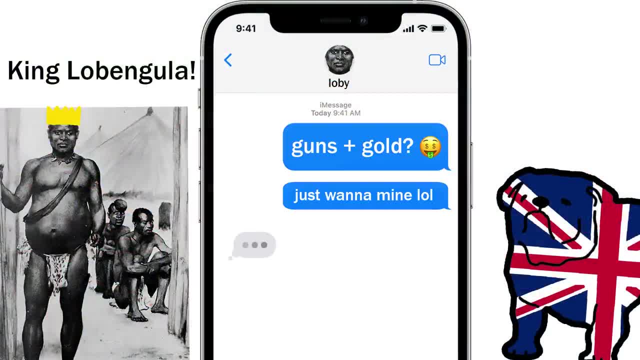 the king they'd give him guns and money if they could mine on the land. And after some thinking it turned out that the Ndebele was the only one who could mine on the land. So the British told the king they'd give him guns and money if they could mine on the land. And after some thinking, 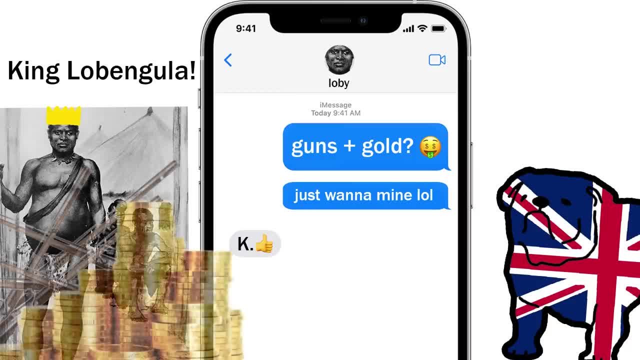 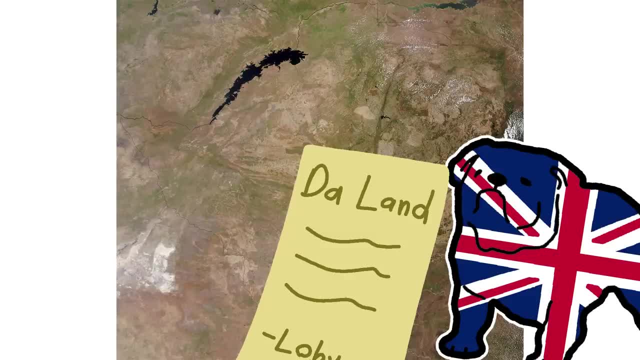 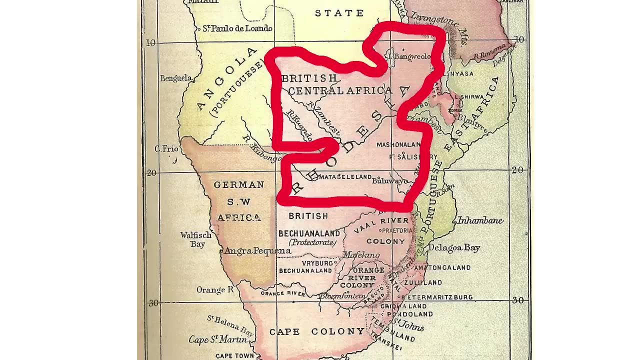 debating, he said: ah, you know what, Screw it. What's the worst that could happen? Except the British didn't actually own this land. One guy named Cecil Rhodes did, and they didn't believe in him, Because now all of this land is called Rhodesia and he's ruling. 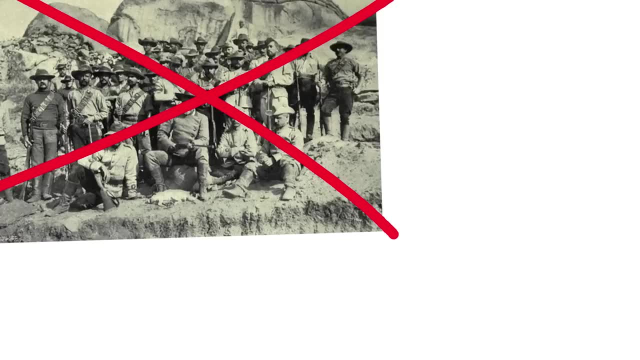 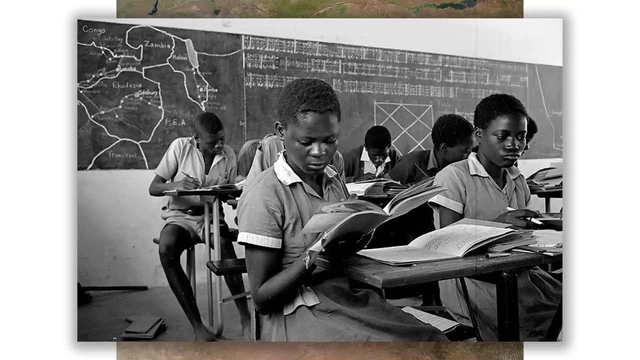 with his divine right to take all the gold from his land. The mining operations actually failed at first, but they still set up some farms to tax food. Rhodesia was a couple of things: It was segregated, it was unequal and it got a little more racist than the average late-night gaming. 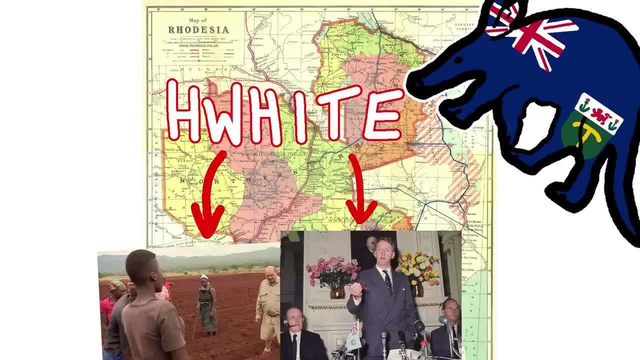 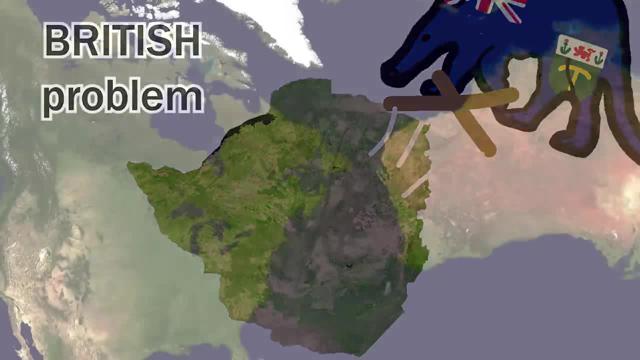 talk. The whites ruled the economy, ruled the country and ruled the land, seizing it from the native Africans, forcing most of them to live on reserves. Only one problem, though: Unlike these countries where the Brits came in such large numbers, they dominated the country. the Brits were the vast minority in Rhodesia, about 50,000 around the 1930s, compared to African numbers in the millions, leading to a country where a tiny fraction of the population of Rhodesians were living on the land. This fraction owned most of the farms, mines, businesses, land and dollar. 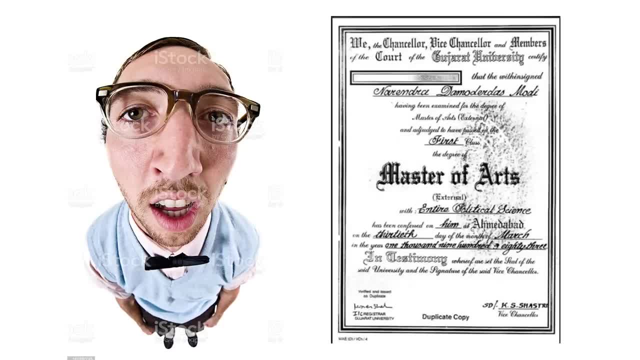 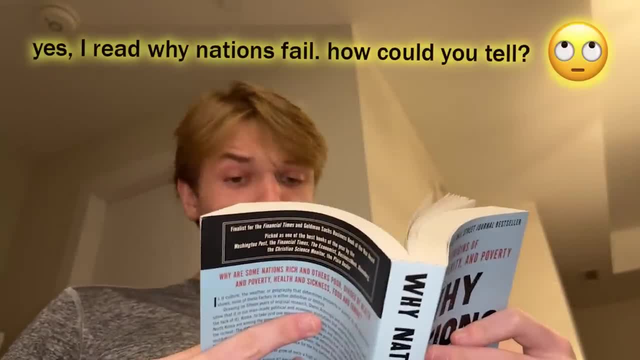 bills. If you want to act like a pretentious political scientist, you could say: Rhodesia was an exemplary case of extractive political and economic institutions set about by an external force for their ad interim growth. Or instead you could say: the Brits took all the 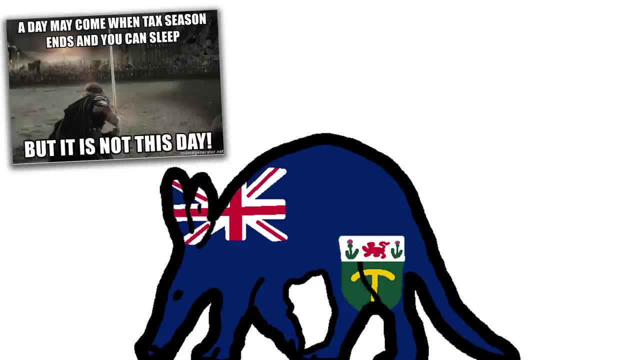 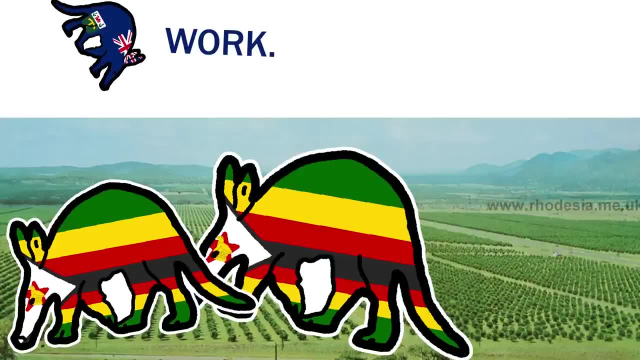 Nobile's things to make some quick cash, Whether from heavy taxes placed on native production, HUD, taxes on every house, or marketing boards set up, who usually took a little bonus for their hard work. Rhodesia was the only country in the world to have such a large amount of money. Rhodesia- 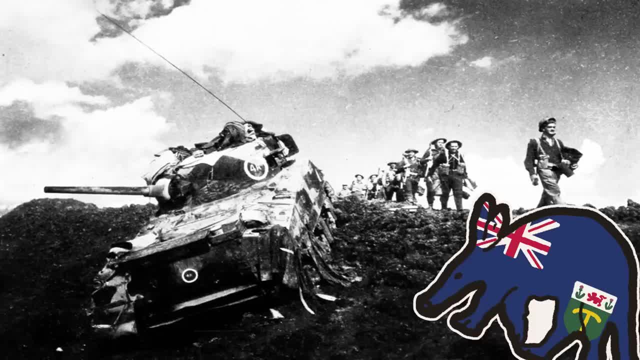 was the only country in the world to have such a large amount of money. Rhodesia was the only country in the world to have such a large amount of money. Rhodesia was more unequal than a Nike sweatshop in Bangladesh And, as World War II started, causing hundreds of thousands of natives. 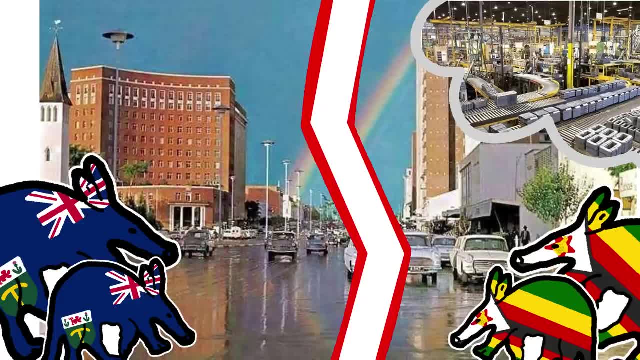 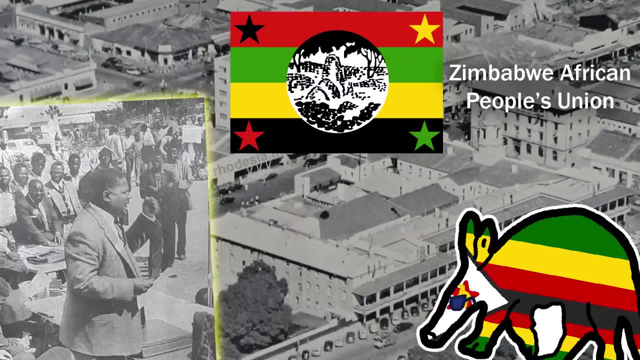 to move to the cities for fancy new manufacturing jobs. tensions only rose between the two groups. The 1950s and 60s saw a rise of militant anti-government groups like the ZAPU and the NDP- this NDP, not the Canadian one. As the groups grew and people kept urbanizing, there were open calls. 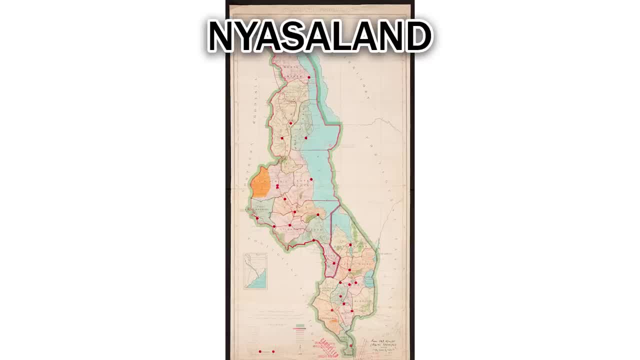 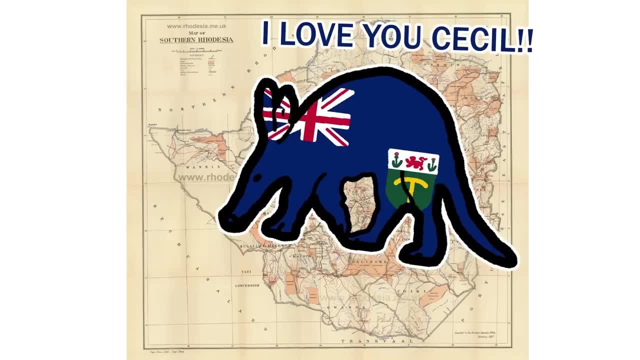 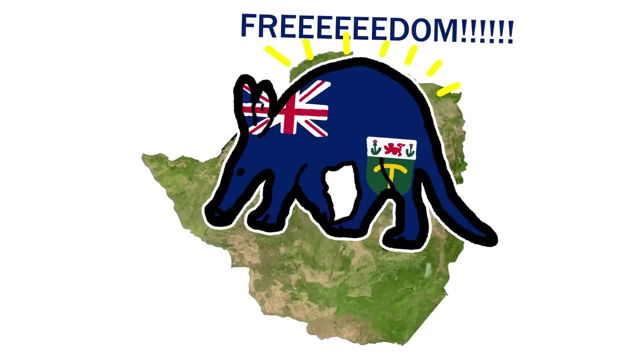 to get rid of the Rhodesian system, And when Nyasaland declared independence in the 60s and then Northern Rhodesia did too, both under African rule, the South wanted to join the party and declared independence from the UK in 1965, instead under a white minority rule. It was inevitable. 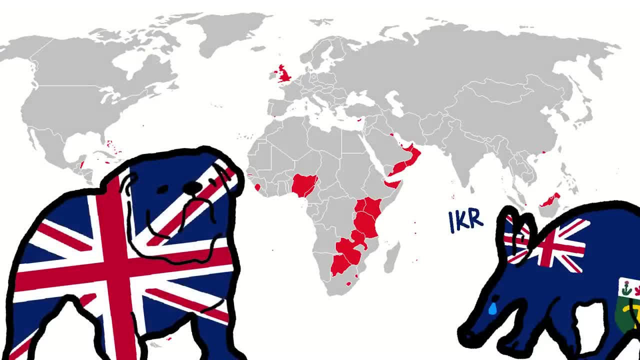 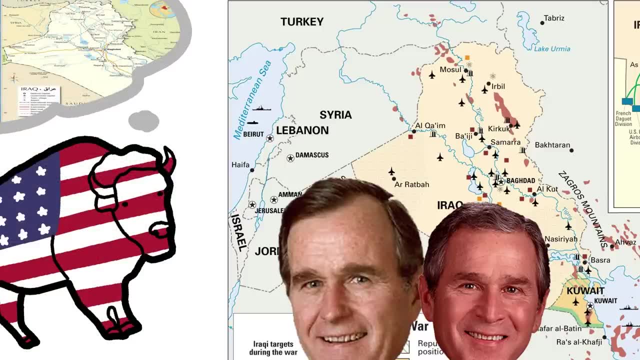 the British Empire was seriously declining and the UK was distancing itself from them. But right after BOOM, the Rhodesian Bush War started and lasted for 15 years. No, not that kind of bush war. it was the Rhodesians vs the Zimbabweans. 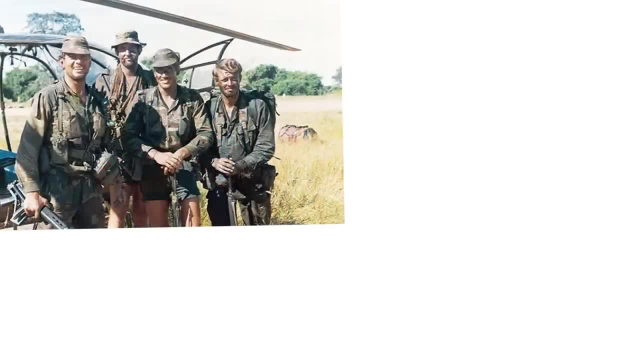 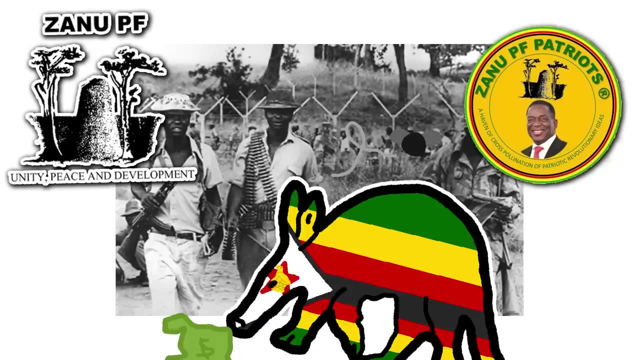 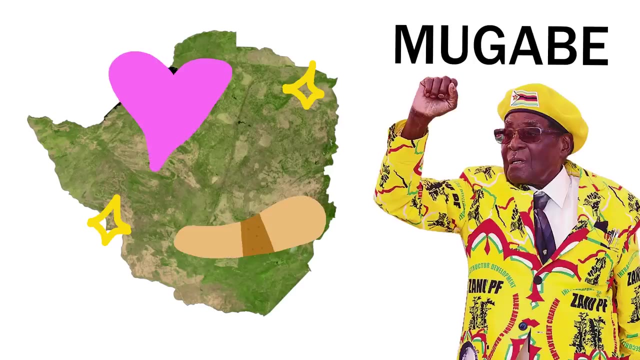 aka whites vs blacks. It obviously caused destruction, countless deaths and embargoes. so when the war was over, won by the ZANU-PF party, the new Zimbabwe was one of the most broken places on earth. Luckily, there was one man who promised to fix Zimbabwe: Robert Mugabe. 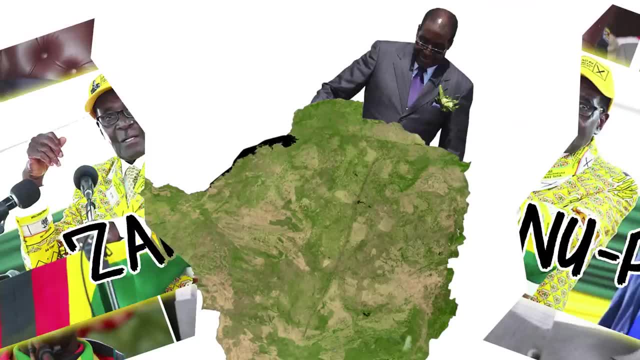 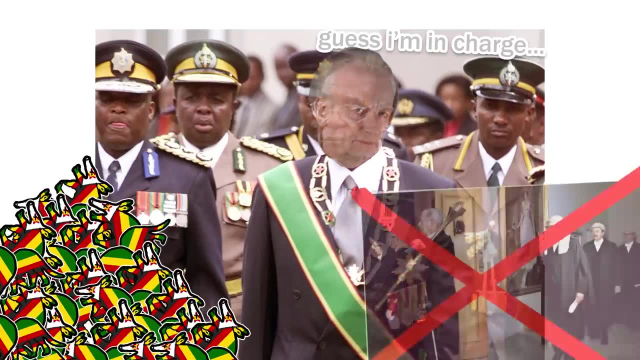 the leader of ZANU-PF. Just kidding guys. this man had no intention of making Zimbabwe a better place. Right after taking over, he killed about 20,000 political opponents and he got rid of the Rhodesian Senate. He was just a tiny bit of a threat to the Zimbabwean people. He was just 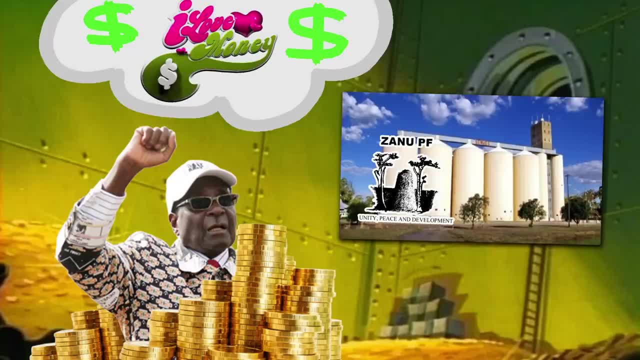 a tiny bit of a threat to the Rhodesian Senate. He was just a tiny bit of a threat to the Rhodesian Senate. He was just a tiny bit of a threat to the Rhodesian Senate. You know, setting up ZANU-PF allies to control newly made state run industries. 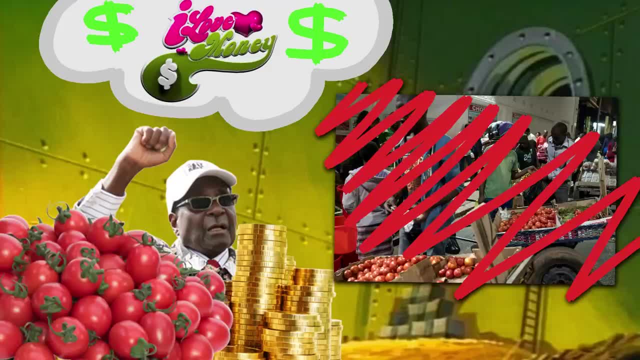 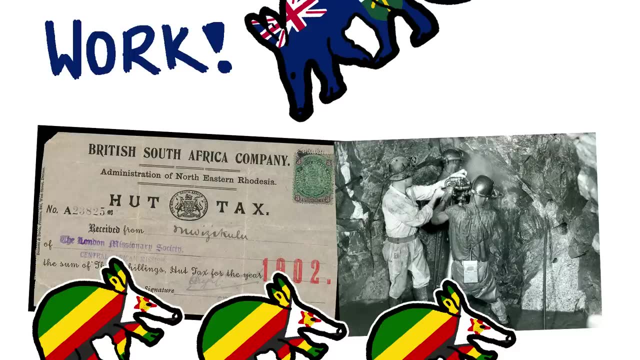 taking over marketing boards and heavily regulating trades, so you had to buy from his party. One could call him a businessman doing business, but many others prefer the term crook. Instead of trying to get rid of these devastating ideas, he wanted to be the man running them. 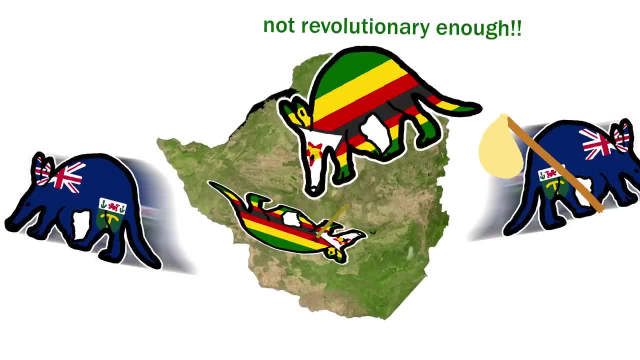 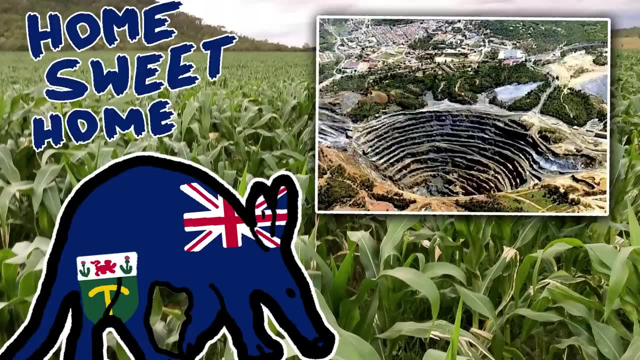 So obviously the old British colonists ran the hell away from this new country, taking much of the money and educated population with them. Some stayed. they still had farms, mines and childhood memories here after all, Plus any type of foreign investment that. 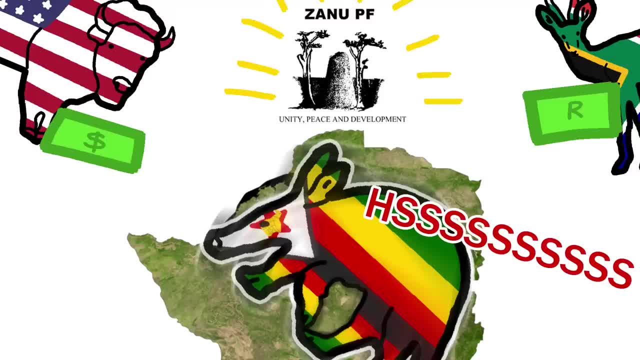 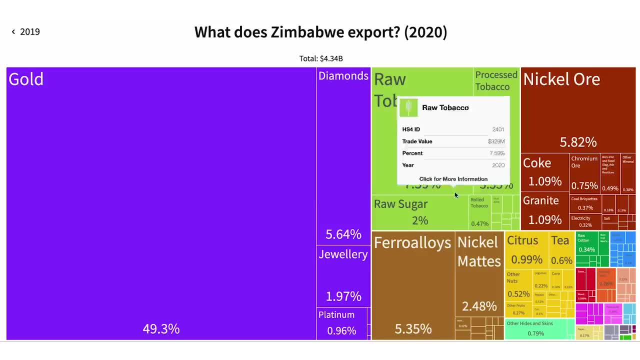 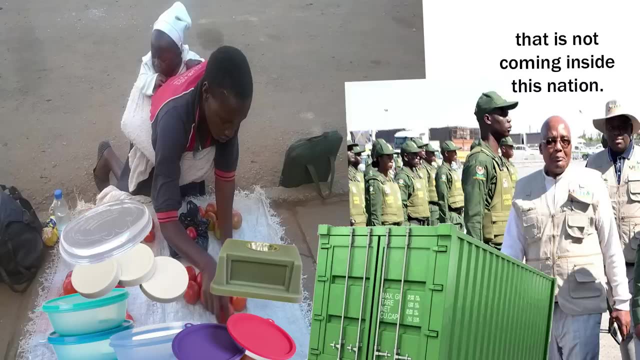 wanted to come back to Zimbabwe was shooed away. ZANU-PF wanted to fix the nation all by itself. So any independent Zimbabwean businessman trying to start up a shop selling I don't know plastic lids couldn't from the heavy subsidies given to ZANU-PF-led industries. high costs from 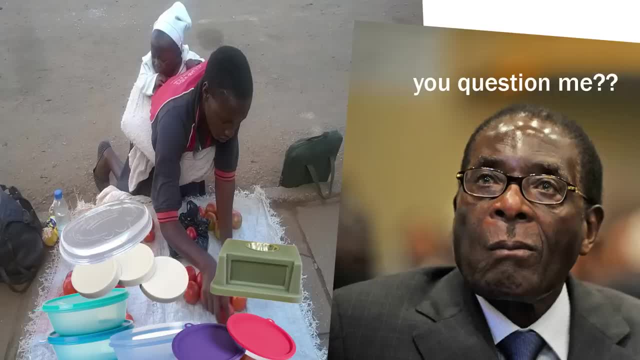 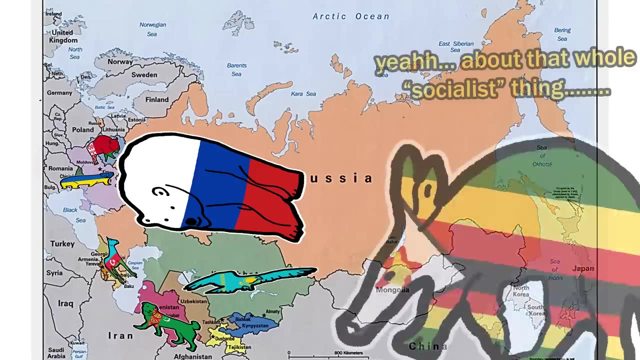 the lack of imports and repression for genuine fear of ZANU-PF power being questioned By the 1990s. this economic system failed. ZANU-PF was the only country in the world that was able to do this After the Soviets collapsed. it wasn't really cool to have a command-based economy. 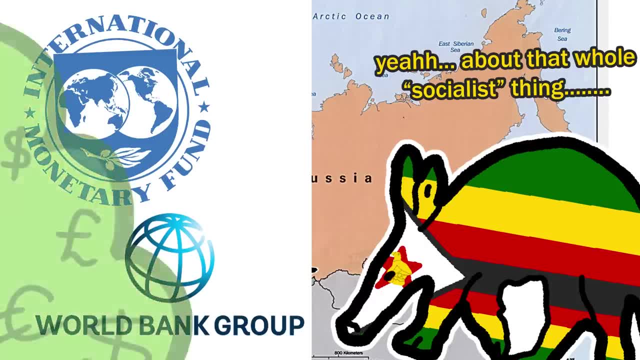 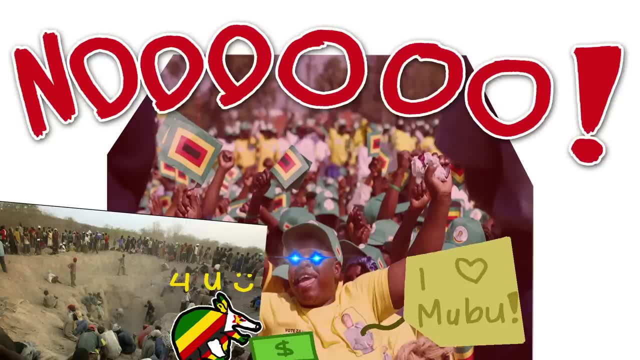 anymore. so they accepted loans from these guys to start a journey to the free market. Nooooooo, said the ZANU-PF supporters, who were the ones controlling all the state-led industries and getting a pretty nice paycheck for their work. so they protested. 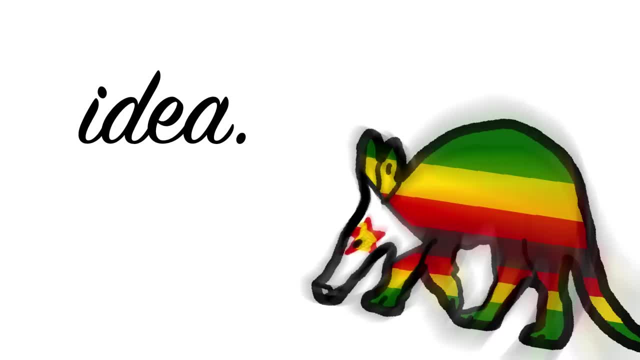 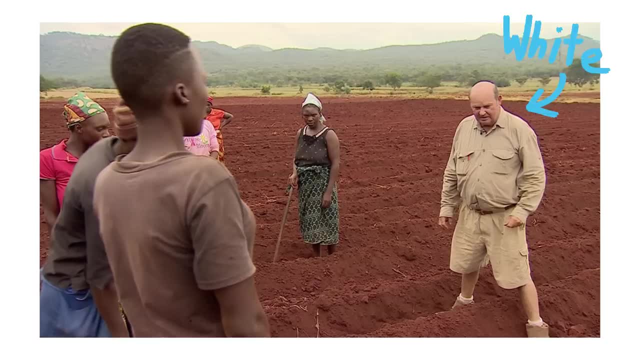 and unrest continued throughout the 1990s. During that whole time, there was an idea, A break-in-case-of-emergency type idea. What if he took all the land from the white farmers and gave it to Blackfriars? Nah, that's too crazy and the debate died down. 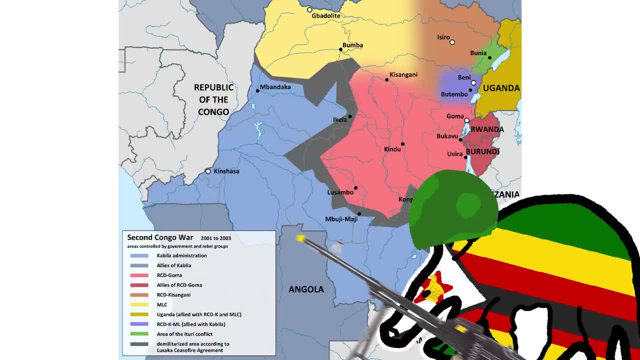 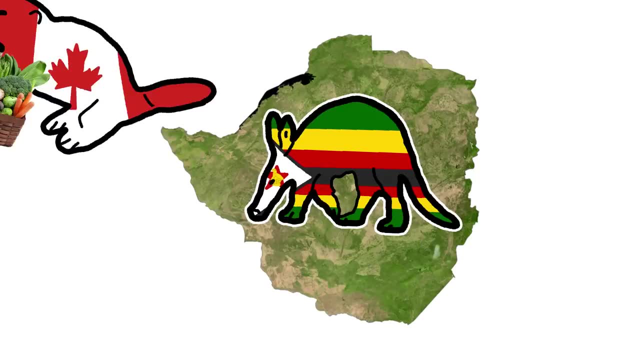 Until 1998 and Zimbabwe went to fight in the second Congo war mainly to protect Mugabe's investments in the country. Turns out that was an incredibly unpopular move and countries cut their aid to Zimbabwe. they cut trade, they cut political ties. 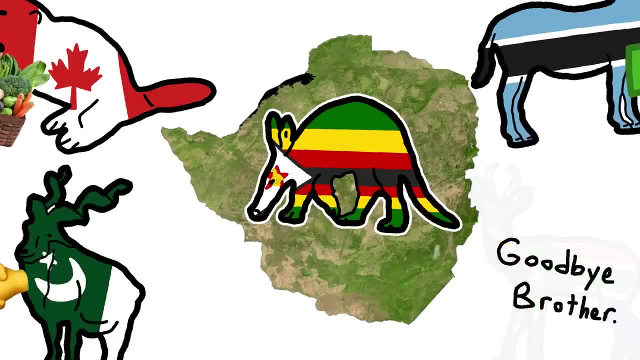 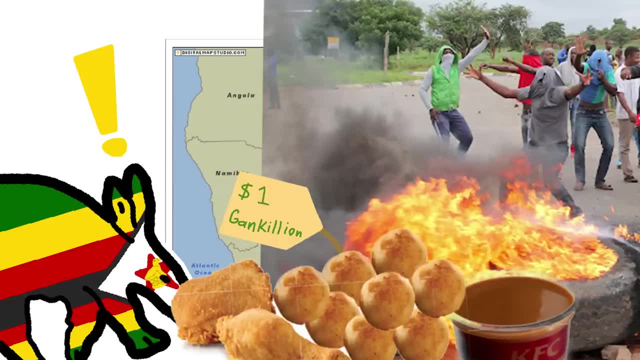 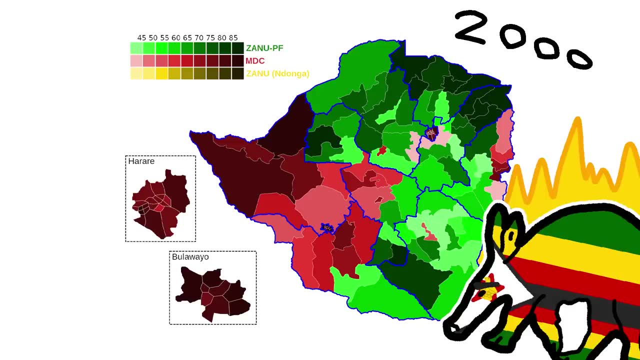 and, most importantly, their old pals South Africa, did all of this too. They were a pariah on the world stage, and it led to deindustrialization, riots over rising food prices, war veterans' demanding land and defaulting on their loans in 2000.. The 2000 election in Zimbabwe was one full of 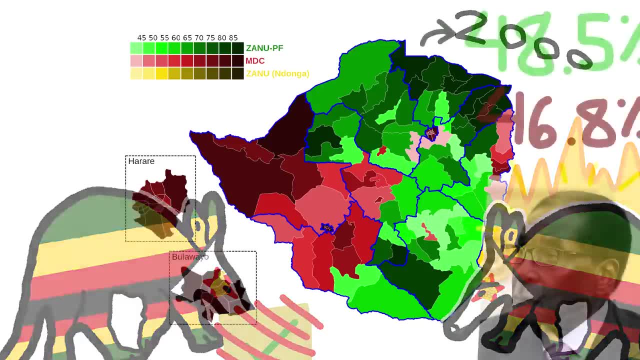 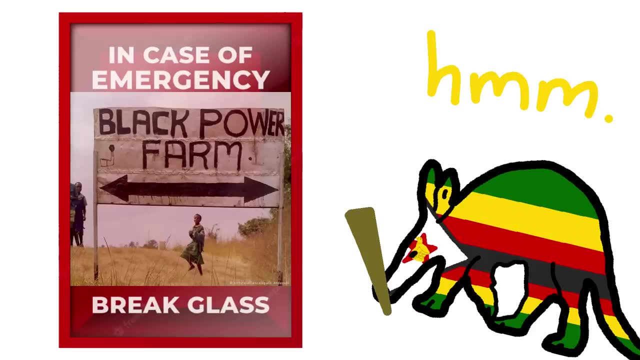 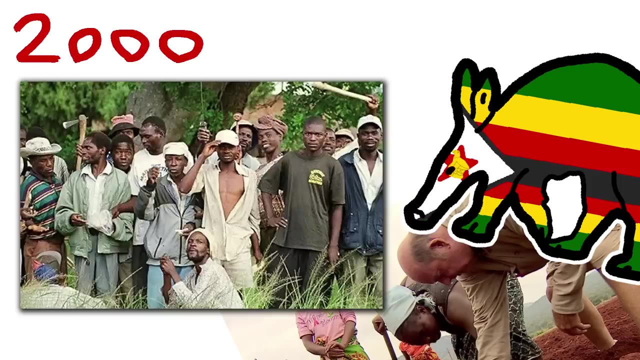 violence, fraud and likely the most important in its history. ZANU-PF won by only a slight margin, with a little help from some certain gunmen. so why not gain some popularity and maybe try that idea out? By 2000,, the government started seizing white-owned land to give to the war veterans. 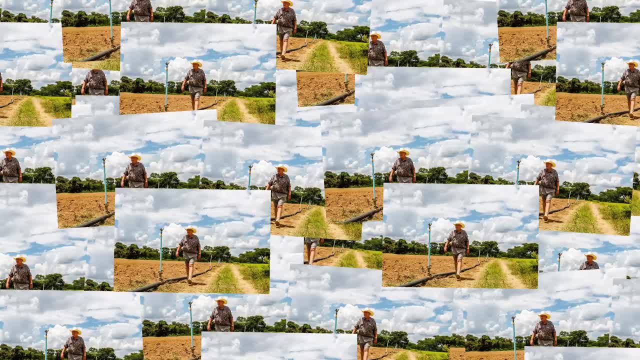 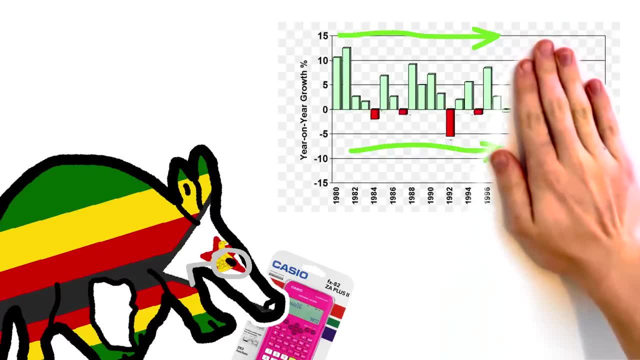 but let's be honest to ZANU-PF elites too, Over 3,000 of them in total, and I think this is going to show the state of the economy best Before 2000,. growing somewhat stable after 2000,. 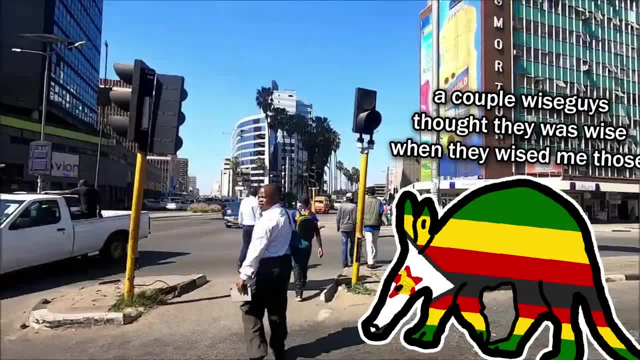 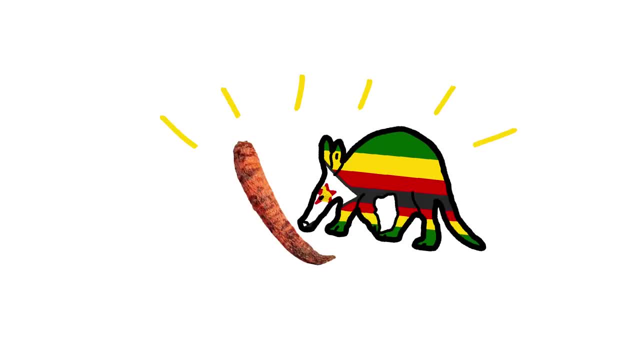 it really took a nosedive. Imagine you lived your whole life in the city and then I grabbed you and threw you on this piece of land and said: farm boy, What would you even do? My guess is you'd be a pretty lousy farmer. and yeah, With the lack of training and dismantling white equipment and 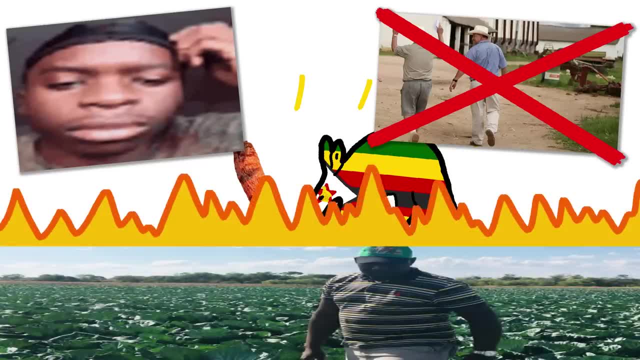 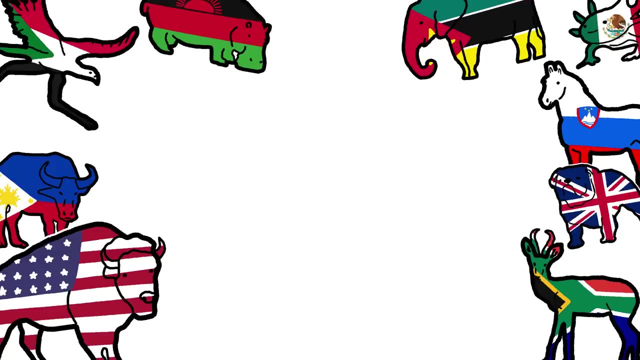 businesses. these new farmers destroyed agriculture in Zimbabwe. Food supplies halved 45% in the years that followed and they couldn't just import the rest. cause, say it together, everybody hates Zimbabwe. Remember this is a country that already lost its trade in. 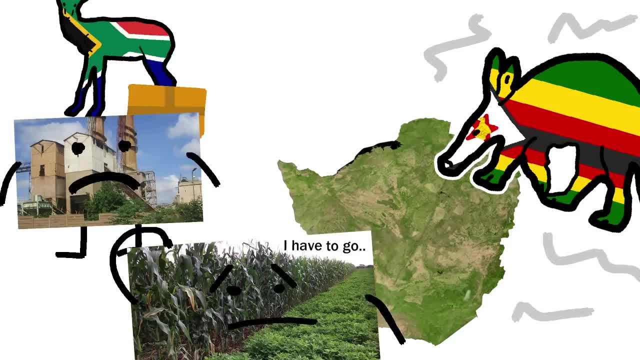 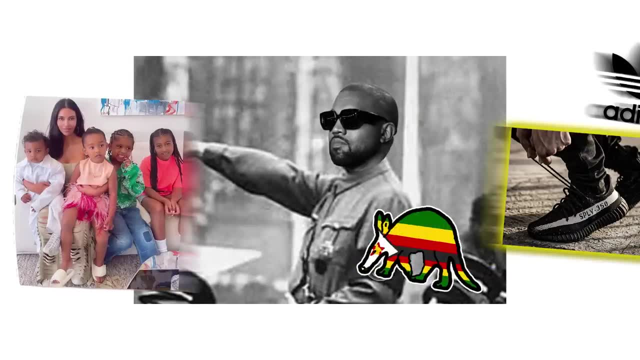 manufacturing. All they had left was farming, and that was collapsing now, too. It's kind of like when Kanye lost his family: all he had left was Adidas, and then he became a Nazi, and he lost Adidas too. Just replace this interview with seizing white farms, and that's the story of 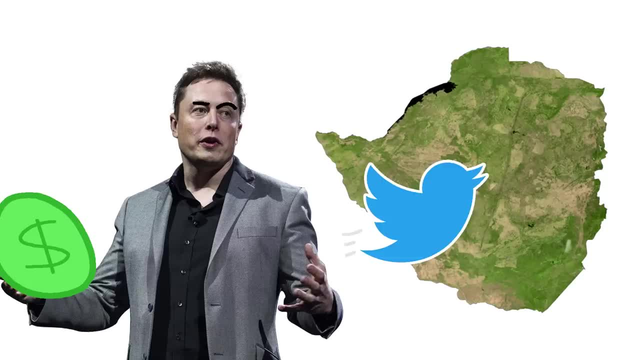 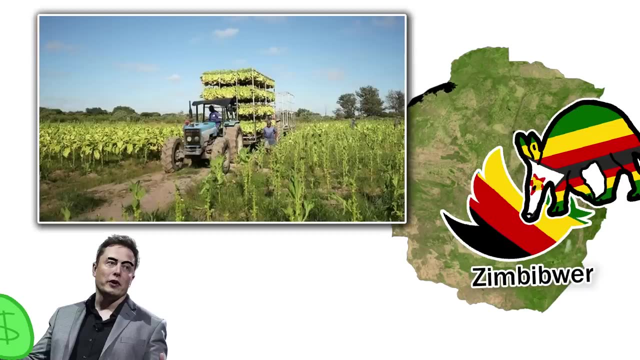 Zimbabwe Businesses completely stopped investing in Zimbabwe when the real world economy was down, realized the government could just snatch their investment from them and shut it down. Well, imagine this with farms and factories instead, And the US and EU put massive sanctions on Zimbabwe, with one of the goals seriously being. 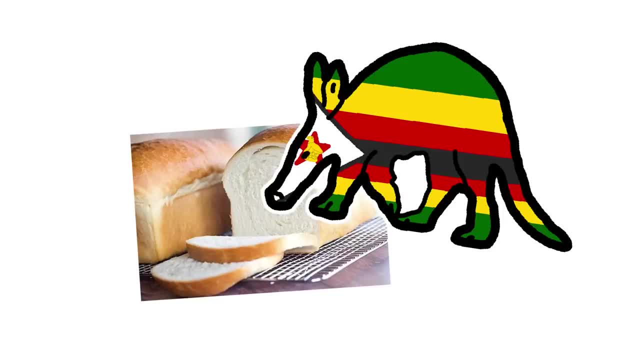 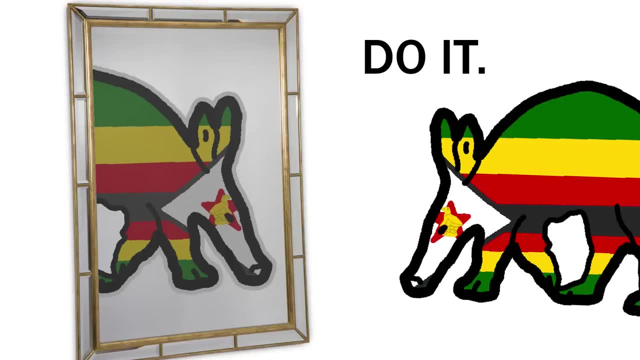 to make the people revolt and overthrow the ZANU-PF government, Food became unaffordable, there was violence and riots in the streets, and the government ran out of money. The only way to pay the elites and veterans was to…. no, don't look at that Zimbabwe. 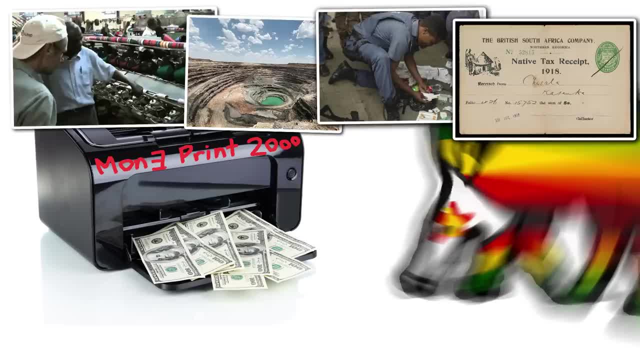 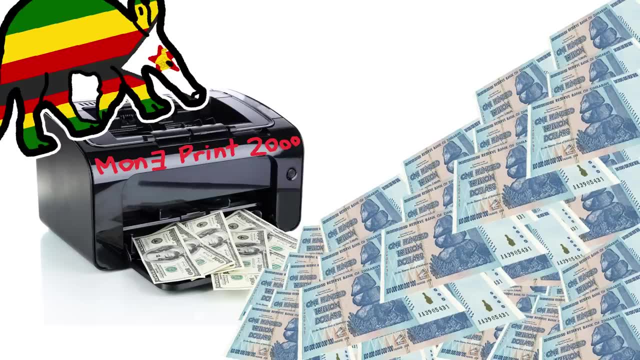 You can do better. Production. diamonds, drug smuggling, taxes, I don't care Anything but that. Oh, but it's so tempting, Maybe just a little bit could do some good cause. swoosh, The government became addicted to printing money. At peak printing in late 2008,. inflation was around 80 billion percent monthly and 90 sextillion percent yearly, but honestly, they stopped measuring. It was so high that everyone was just honestly making these stats up. They printed so much money that the paper it was printed on was way more valuable than 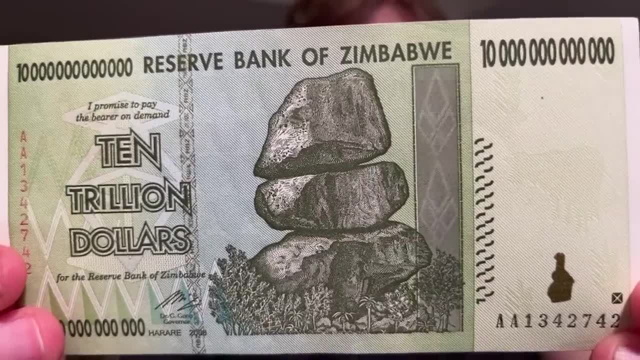 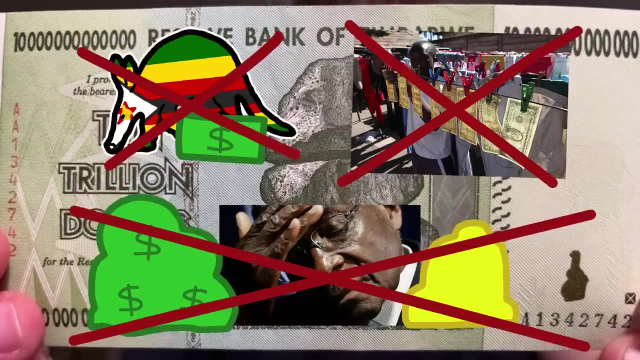 the dollar itself, leading to things like the 10 trillion dollar bill and the hyperinflation, wiped out everybody's savings, destroyed any businesses' savings and obliterated the government's savings. The black market was the only realistic way to buy food goods and to find any work with.